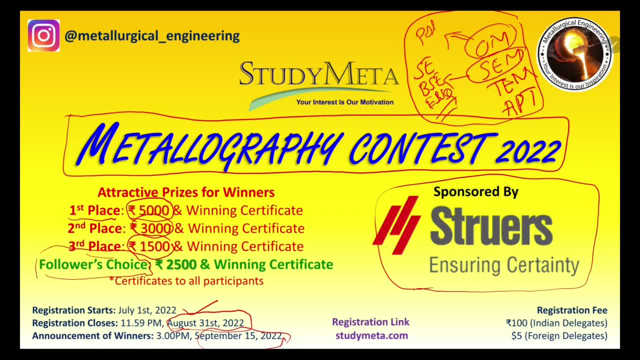 upload all the images that we have. this that we will. this received in this event, so we will post on our social media. so this, whichever image will like highest this likes, so they will get this 2500 rupees a price. so I would like to invite. 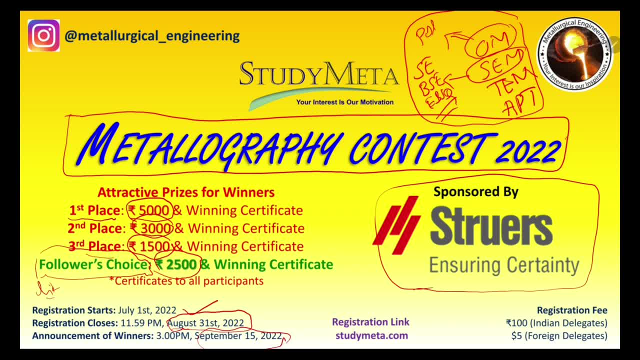 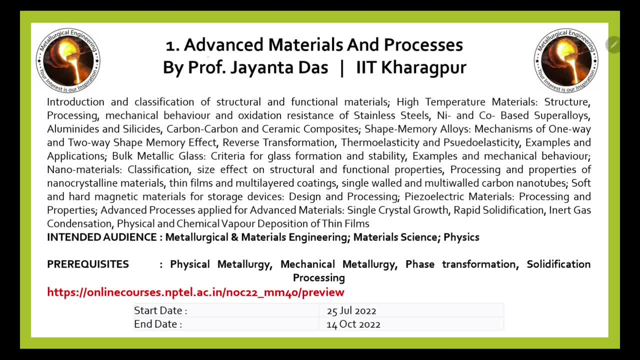 you to to participate in this event and make this as a grand success. so let's go to the main part of the video. so the first course is advanced material- advanced materials and processes by Professor Jan Tadas from IIT Kharagpur. so in this course we will going to study the introduction and classification of 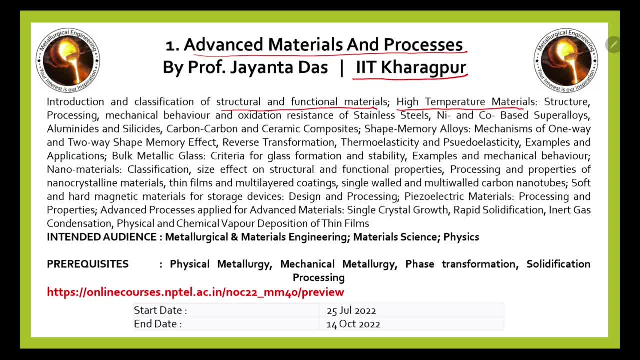 structural and functional material high temperature- these materials structure processing, mechanical behavior and oxidation resistance. and the material high temperature, these materials structure processing, mechanical behavior and oxidation resistance of stainless steel, nickel and cobalt based super alloys, aluminides, silicide, carbon, carbon and ceramic composite safe memory alloys. mechanism of this one way. 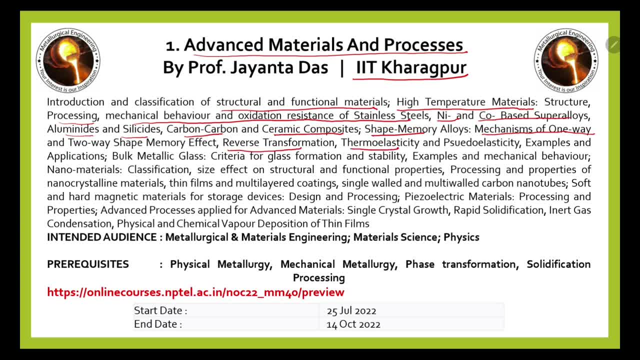 and two way safe memory effect, reverse transformation, thermoelasticity, pseudo elasticity. examples and application: bulk metallic glasses. so these are the things you are going to study in this course. so the main part is that that intended audience is metallurgical and materials engineering and material science students and physics students, and pre prerequisites for this course you have. 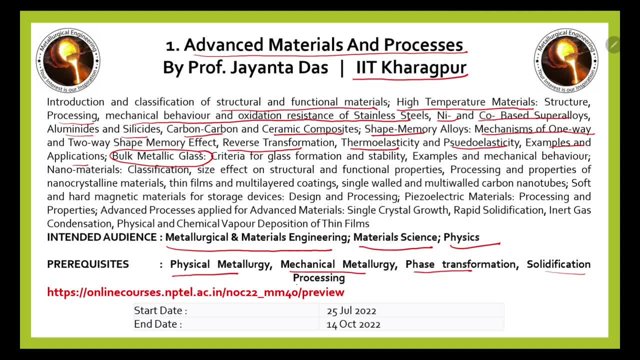 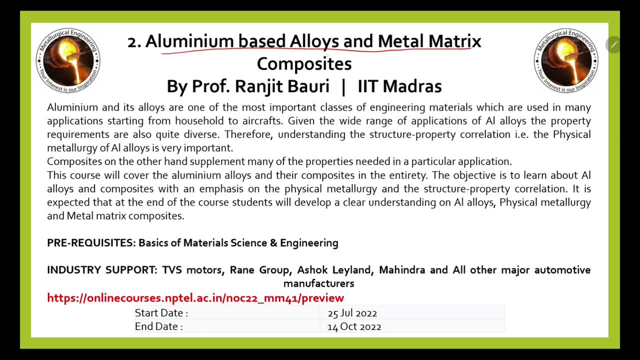 some knowledge of physical metallurgy, mechanical metallurgy, phase transformation and solidification processes. so these are. so this is the link you can access and this course will start on 25th July and end date is 14th October. so the second course in this list is aluminium based alloys and metal. 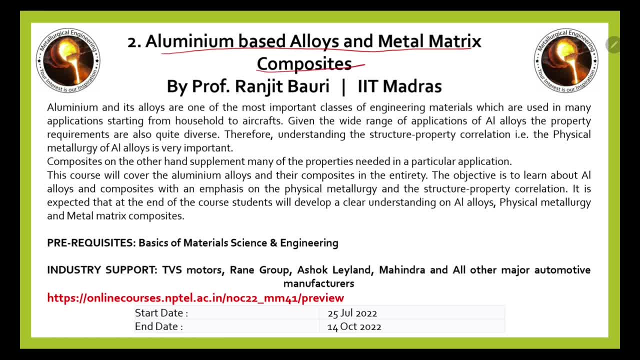 matrix composite. this course is offered by Professor Ranjit Bauri from IIT Madras. so in this course you are going to study about the aluminium alloys and how this has uh used in this metal matrix composite. so basically the prerequisite for this course uh is like you have some information about basic uh, this material science and engineering, and also 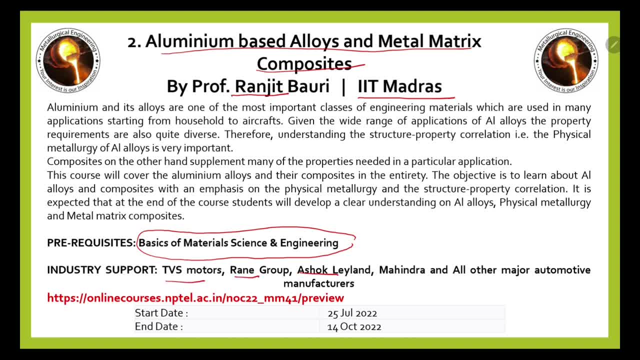 industry uh support like tbs motor, dana group, asok landmines and all major manufacturing automotive component. uh, these manufacturers also attend this course. so the same start date is on the 5th of july and 14th october is the last date of this course. uh, third course is bonds and bands in. 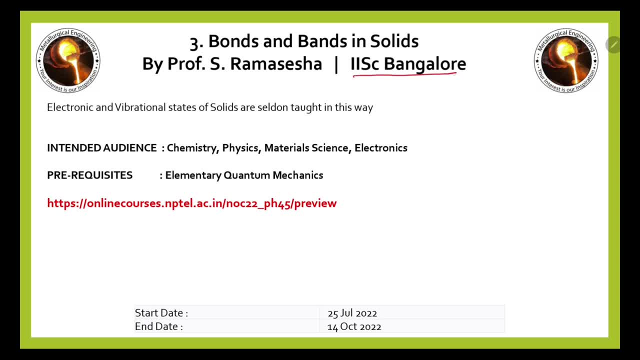 solids. this is offered by professor s ramesa from isc bangalore. so in this course you are going to study what electronic and vibrational states of solid are certain taught in this way. so in this survey, and intended audience is like chemistry, physics, material science and electronics students. 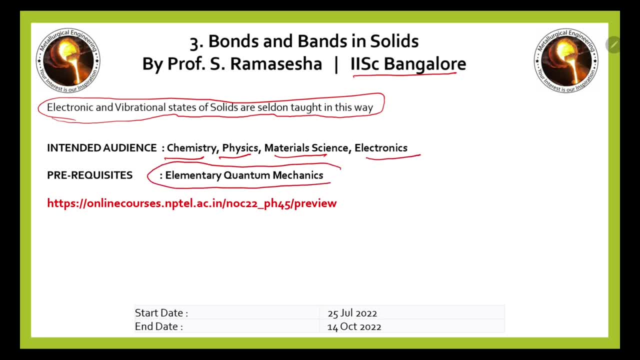 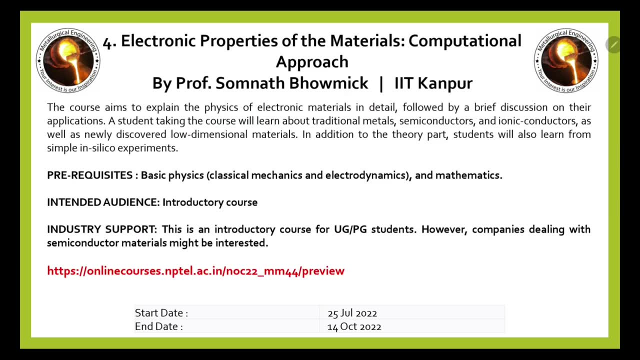 and prerequisites for this course. you have some knowledge of elementary quantum mechanics. so the same start date is 25th of july now. next course in this list is electronic property of the materials, computational approach. so this course is offered by a professor, somnath. professor somnath from iit kanpur. so the 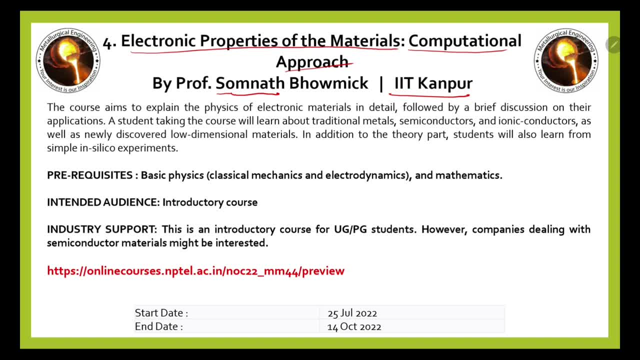 the course aims to explain the physics of electronic materials in detail, followed by a brief discussion on their applications. a student taking this course will learn about a traditional metal, semiconductor and ionic conductor, as well as newly discovered low dimensional materials. so the prerequisites for this course: you have some knowledge of basic physics, like classical 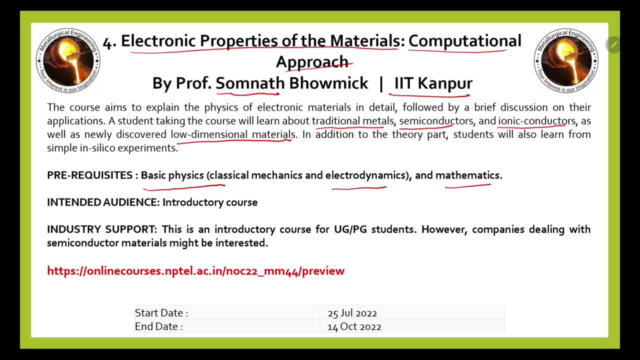 mechanics and electrodynamics and mathematics. so also this is an introductory course, and also the industry. this is introductory course for ugpg student. however, companies dealing with semiconductor materials might be interested. so again, this course is started on 25th july. next course in this list is elementary astrology of quantitative metallurgy. 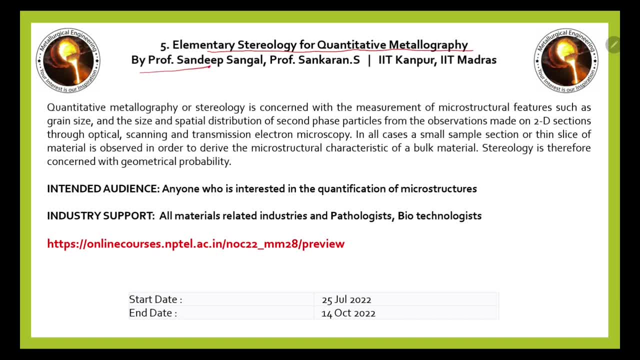 so this course is offered by professor sandeep sangal and professor sankaran s from iit kanpur and iit madras. so in this course you are going to learn about, quantitative metallography, or astrology, is a concern with the measurement of microstructural features such as grain size and the size and 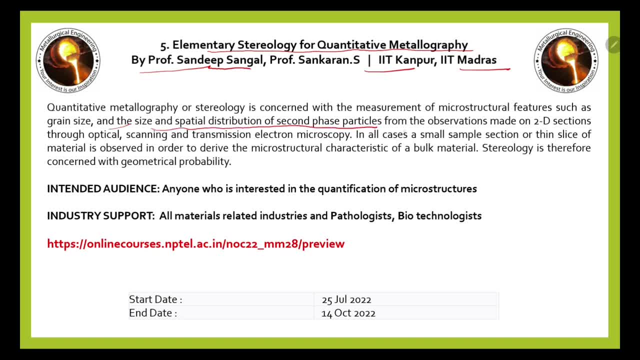 spatial distribution of second phase particles from the observation made on a 2d section through optical scanning and transmission electron microscopy. so in all cases a small sample section are thin-skinned particles. slice of material is observed in order to derive the microstructural characteristics of a bulk. 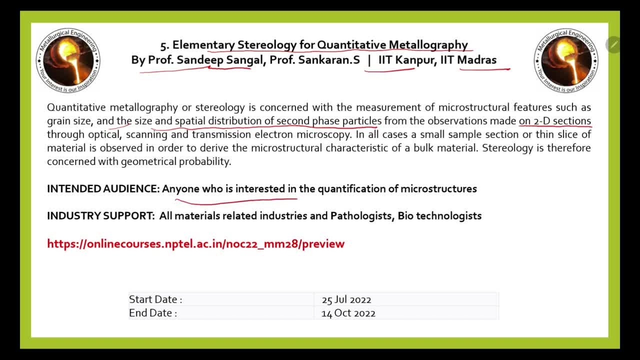 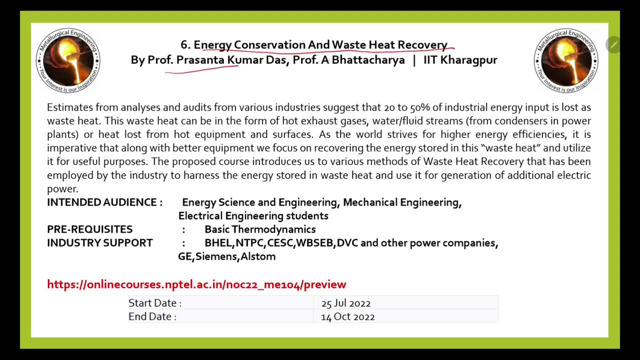 material. so intended audience: anyone who is interested in quantification of microstructure, also all materials related industry and pathologist, biotechnologist can attend this course. this course is estimates from analysis and audits from various industries suggest that 20 to 50 percent of industrial energy inputs is lost in base heat. So this base heat can be in the form of hot exhaust gases. 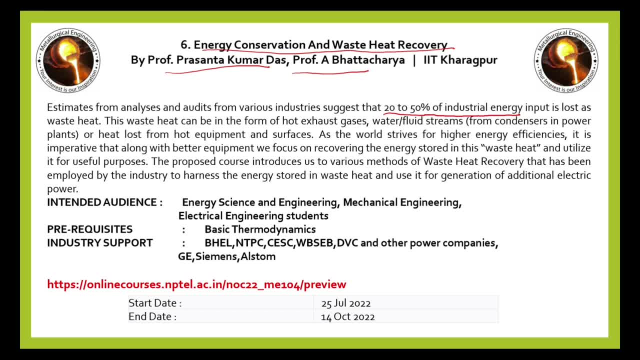 water, fluid streams or heat lost from hot equipment and surfaces. So, as the world strives for higher energy efficiency, it is imperative that, along with better equipment, we focus on recovering the energy stored in this base heat and utilize it for useful purposes. So in this course, 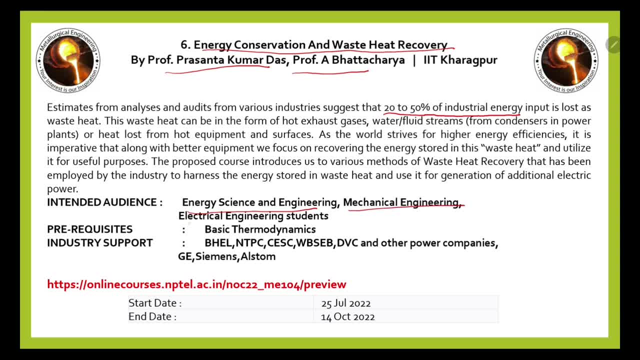 energy science and engineering, mechanical engineering, electrical engineering students. So these prerequisites for this course is you have some knowledge of basic thermodynamics and also industry person like Bale, NTPC, CESC, WBSAB, DBC and other power companies like GE, Siemens. 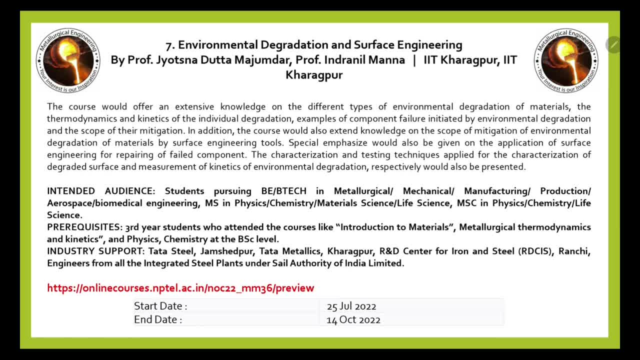 can also attend this course. So next course in this list is environmental degradation and surface engineering. This course is offered by Professor Jyotsana Rekhita Majundar and Professor Indranil Manna from IIT Kharagpur, So this course would offer an 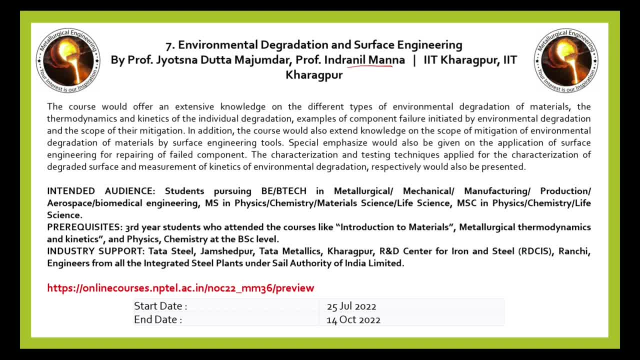 extensive knowledge on the different types of environmental degradation of materials, the thermodynamics and kinetics of individual degradation, examples of component failure initiated by environmental degradation and scope of this mitigation. So, in addition, the course would also extend knowledge on the scope of mitigation of environmental degradation of materials by 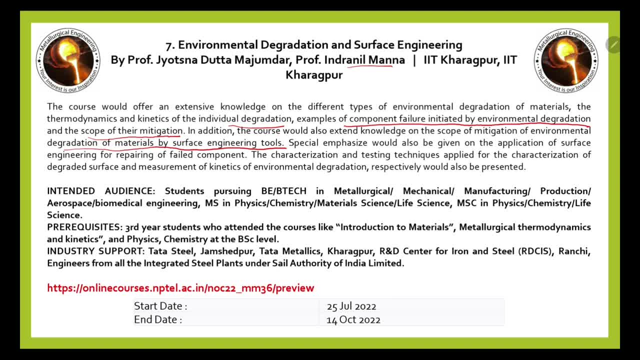 surface engineering tools. So in terms of environmental degradation and the scope of environmental degradation of materials by surface engineering tools. Attended audience like student pursuing BE, BTech in Metallurgical, Mechanical Manufacturing, Production, Aerospace, Biomedical, MS in Physics, Chemistry, Material Science, Life Science, MSc in Physics, Chemistry, Life Science. 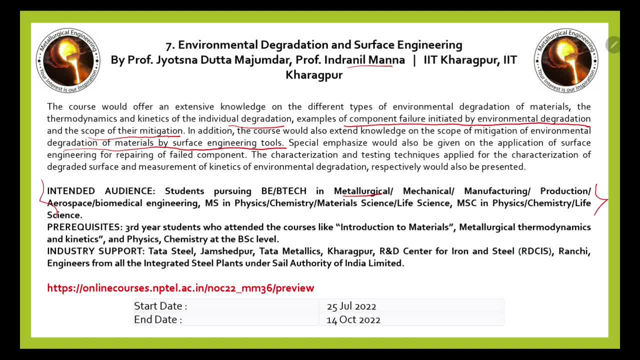 So all the students who are having this one, they can attend this course. And the prerequisites- like third year student who attended the course, like Introduction to Materials, Metallurgical Thermodynamics and Kinetics and Physics, Chemistry at the BSc level. So these are the prerequisites of this course. 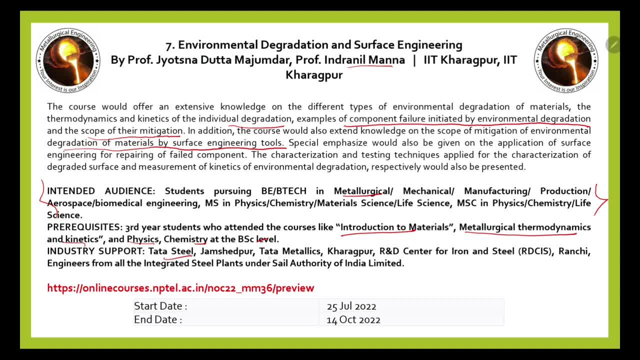 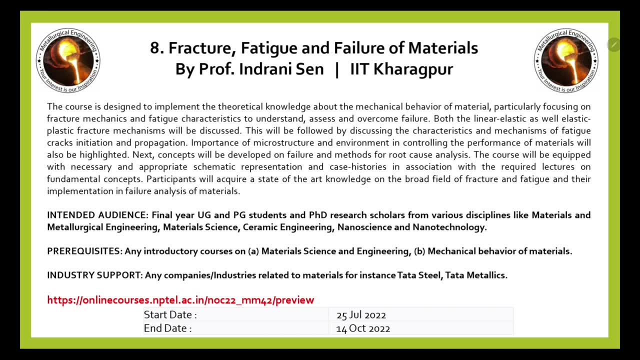 And industry support, like TATA Steel Jamshedpur, TATA Metallics Kharagpur, R&D Centre of Iron and Steel, RACHI. So engineers from all the integrated steel plants under sale they can attend this course. Next course in this list is Fracture, Fatigue and Failure of Materials. 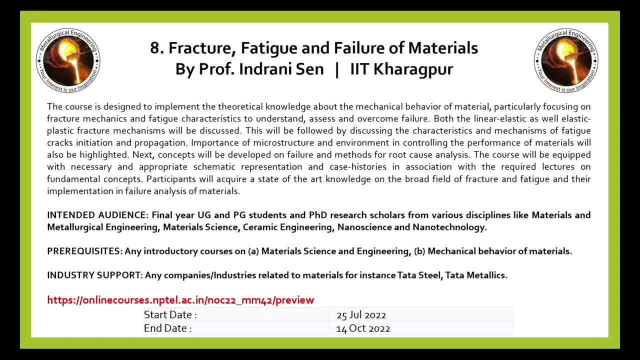 It is offered by Professor Indrani Singh from IIT Kharagpur. So this course is designed to implement the theoretical knowledge about the mechanical behaviour of materials, Particularly focusing on structure mechanics and fatigue characteristic, to understand, assess and overcome the failure. 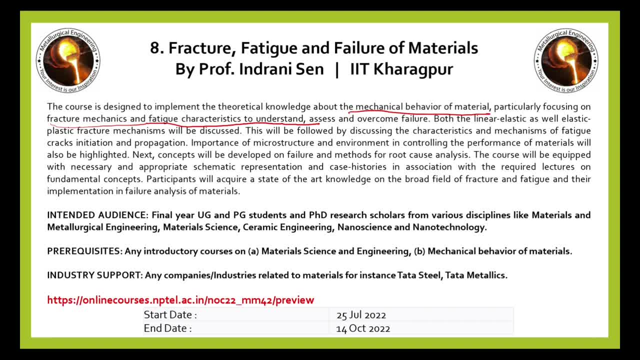 So both the linear, elastic as well as elastic plastic structure mechanics will be discussed in this course. This will be followed by discussing the characteristics and mechanisms of fatigue crack initiation and propagation. Importance of microstructure and environment in controlling the performance of materials will also be highlighted. 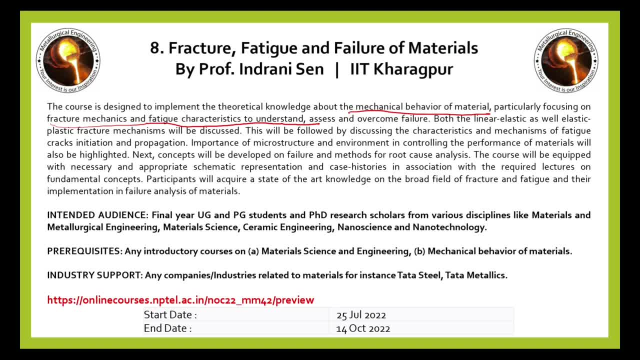 So next is concepts will be developed in failure And methods for root cause analysis. So the course will be equipped with this necessary and appropriate schematic representation and case history in association with the required lectures on the fundamental concepts. So the intended audience for this course is final year UG and PG student and PhD research scholar from various disciplines like materials and metallurgical engineering, material science, ceramic engineering, nanoscience and nanotechnology. 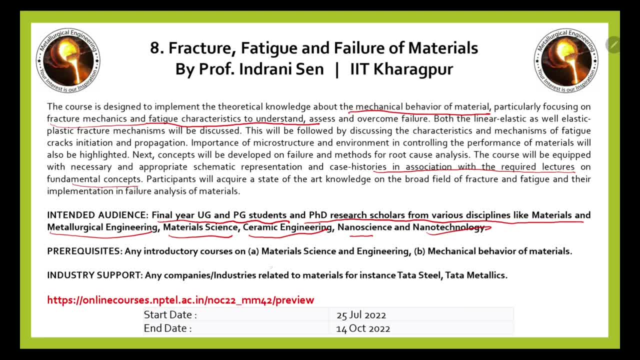 So the prerequisites of this course: You have some knowledge of basic material science and engineering course and mechanical behaviour of these materials. So industry, so any company, industry related to materials, for instance Tata steel, Tata metallics, they can attend this course. So ninth course in the list is fundamentals and application of dielectric ceramics. 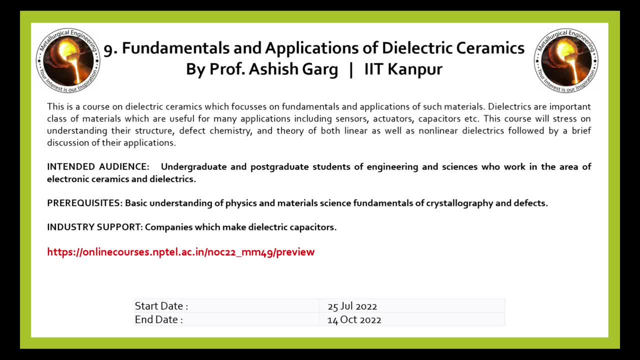 It is offered by Professor Ashish Garg from IIT Kanpur. So this is a course on dielectric ceramic which focuses on fundamentals and application of such materials. So dielectrics are important cross-off materials which are useful for many application, including sensors, actuators, capacitors. 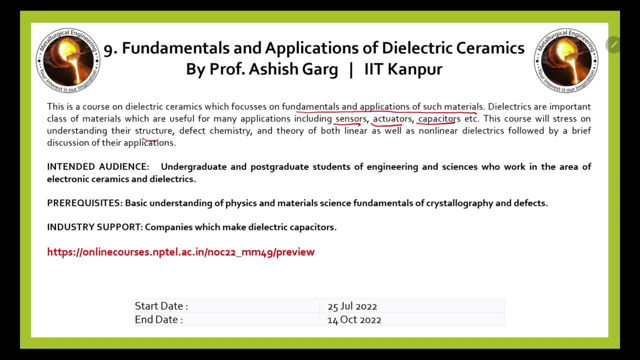 So this course with a stress on understanding the structure, defect, chemistry and theory of both linear as well as nonlinear dielectric, followed by a brief discussion about their applications. So the intended audience for this course: undergraduate and post graduate student of engineering and science who work in the area of electronic, ceramic and dielectrics. 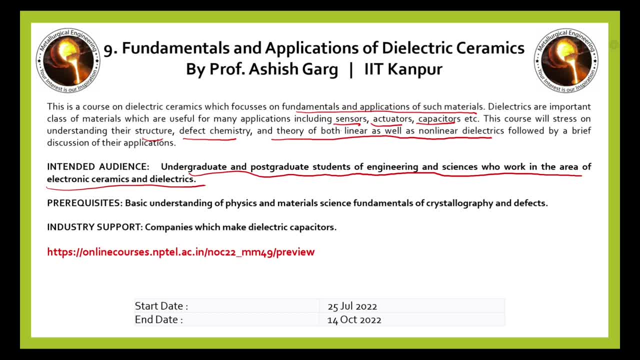 So basic understanding, understanding of physics and material science, fundamentals of crystallography and defects are required for this course, And companies which make dielectric capacitor also attend this course. Tenth course in this list is Fundamentals of Electronic Device Fabrication. This is: 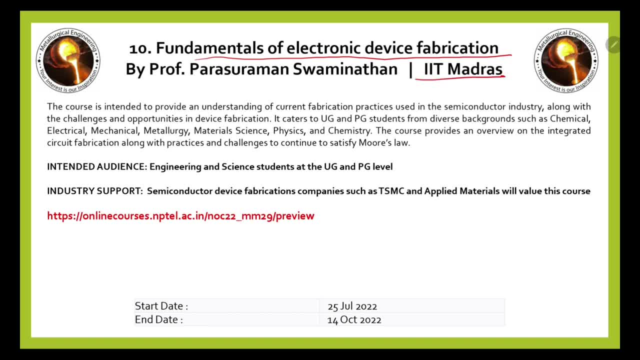 offered by Prof Swaminathan from IIT Madras. The course is intended to provide an understanding of current fabrication practices used in the semiconductor industry, along with the challenges and opportunities in the device fabrication. So intended audience is engineering and science students at UG and PG level, and also semiconductor device fabrication companies such as TSMC. 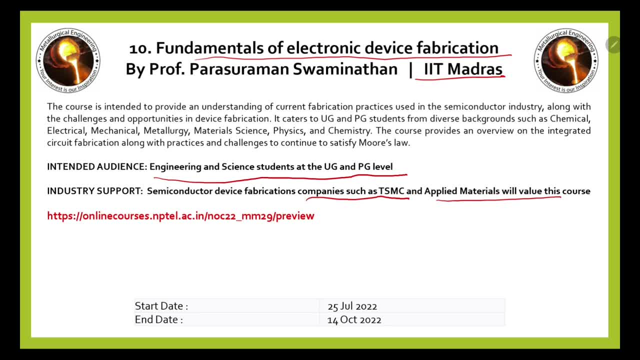 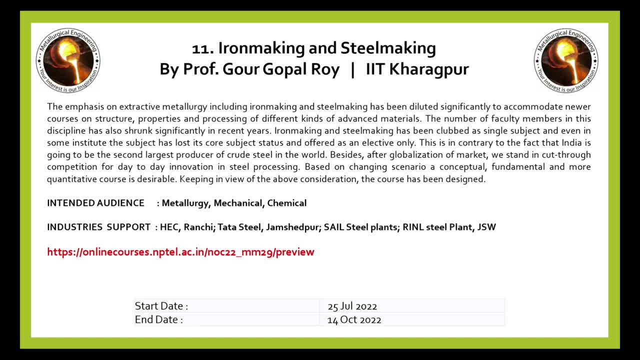 and applied materials will value this course. Eleventh course in this list is Iron Making and Steel Making. So the emphasis on the on extractive metallurgy, including iron making and steel making, has been diluted significantly to accommodate a newer courses on structure, property and performance. 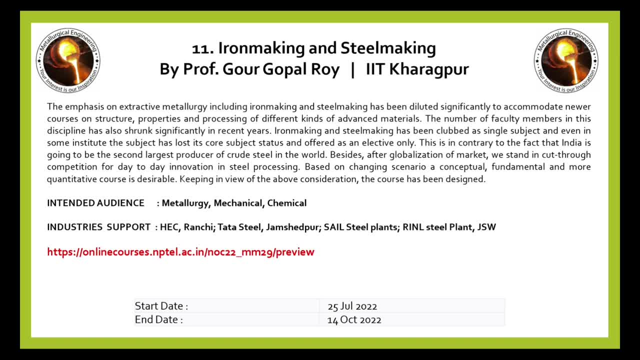 So the emphasis on class, structure properties and possibilities in the device fabrication processing of different kinds of advanced materials. The number of faculty member in this discipline has also shrunk significantly in recent years. So iron making and steel making has been clubbed as a single subject, and even in some institute the subject has lost its core. 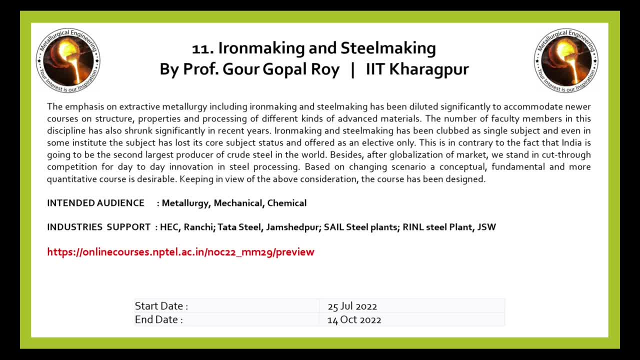 subject status and offered as an elective only. So this is a contrary on the fact that India is going to be the second largest producer of the crude steel in the world. Besides, after globalization of market, we stand in cut through competition by day by day innovation in steel processing. So 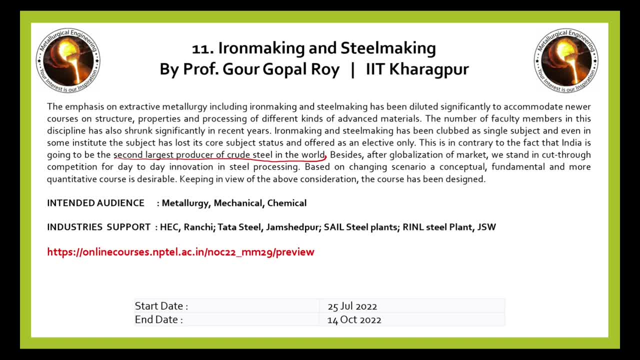 based on changing scenario, a conceptual, fundamental and more quantitative course is desirable. So, keeping in the view of the above consideration, the course has been designed and if you are interested and if you are working in steel industry, this particular course will be useful for you And if someone is looking to make a career in steel industry and how this 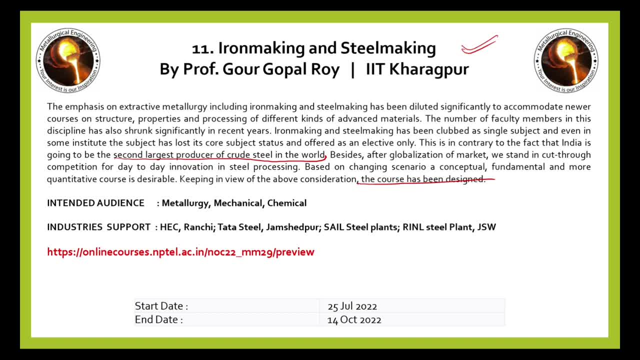 how this new technologies can change can make a change in steel industry and to bring down the carbon dioxide this reductions. So this particular course will be useful for you to make these concepts So. intended audience is metallurgy, mechanical and chemical engineering students and industry support. 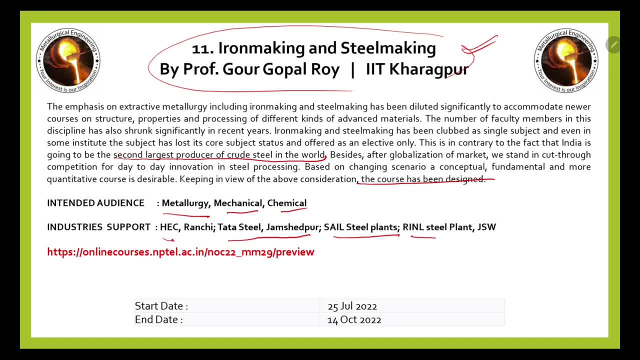 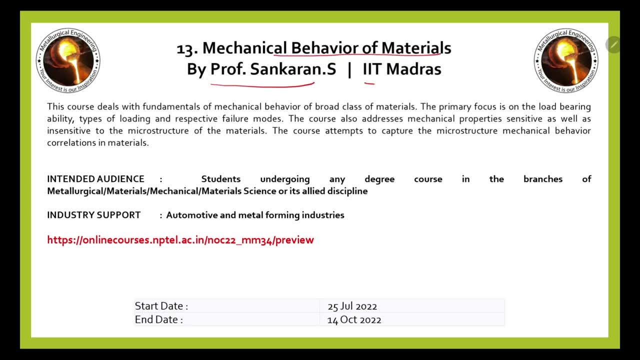 like HEC, RACHI, TATA, Jamset, Purcell steel plants, RINL plants, CSW. they all are highly recommended to attend this course. Thank you. Next in this list is mechanical behavior of materials by Professor Sankrant from IIT Madras. 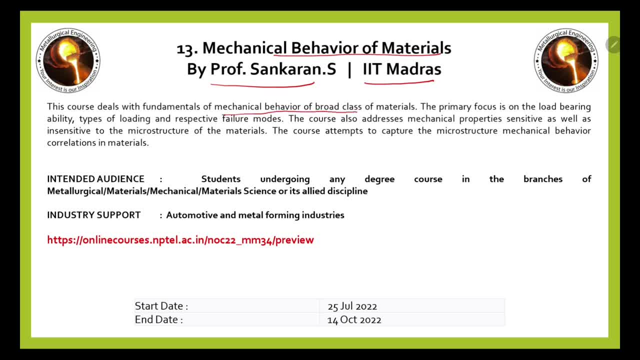 So this course deals with the fundamental and mechanical behavior of broad class of materials. The primary focus is on the load bearing ability, types of loading and respective failure modes. So the course also addresses mechanical properties sensitive as well as insensitive to the microstructure of the materials. The course attempts to capture the microstructural 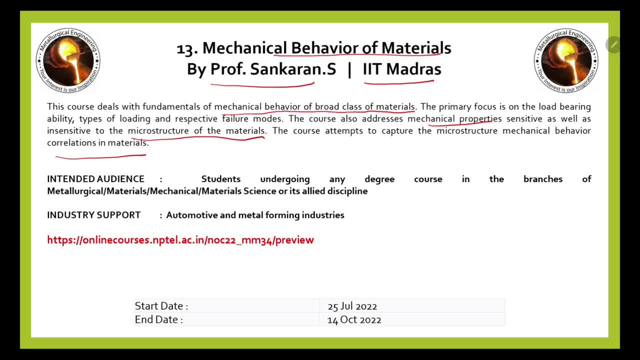 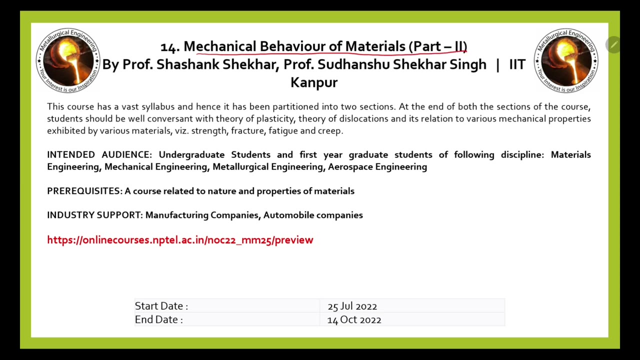 mechanical behavior. So student undergoing any degree courses in the branch of Metallurgical Materials- Mechanical Material Science are it's disciplines- are recommended to attend this course, and also from automotive and metal forming industries persons can also attend this course. Next in this list is mechanical behavior of material, par-2, that course is offered by: 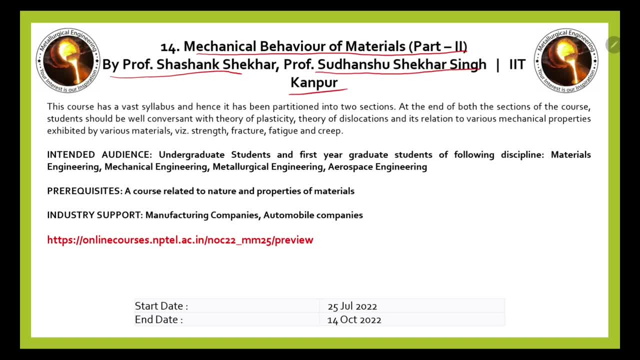 Professor Sasam Sekhar and Professor Sudhanshu Sekhar sing from IIT Kanpur, so this course has a vast syllabus and hence it has been partitioned into the two sections. at the end of both the sections of the course, students should be well convergent with theory. 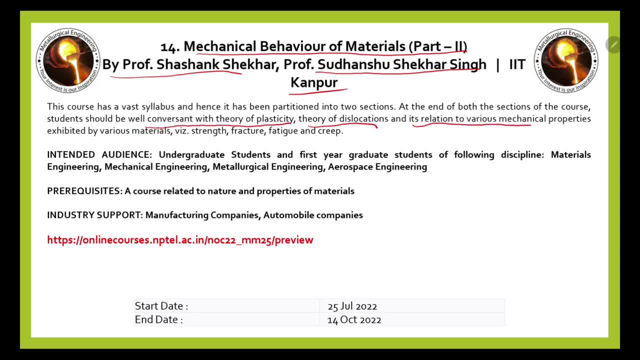 of plasticity, theory of dislocation and its relation to various mechanical properties exhibited by various materials, like strength, fracture, fatigue, creep. so the intended audience for this course is undergraduate student and the first year graduate student of the following disciplines: materials engineering, mechanical engineering, metallurgical engineering and. 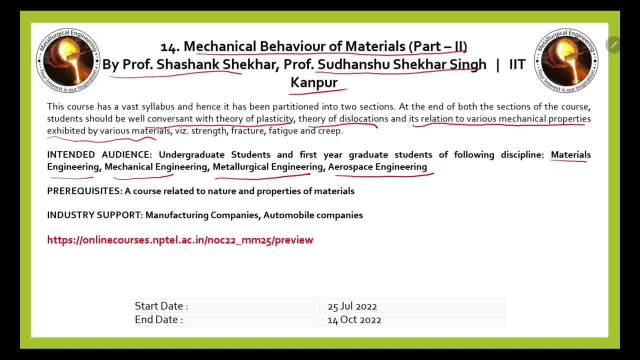 aerospace engineering. so the prerequisites of the course, a course related to nature and property of material, like structure of materials. so these are the course you have to know before attending this course and the manufacturing companies- automobile companies are highly recommended for attend this course. next course in this course, in this list, is nanotechnology science and 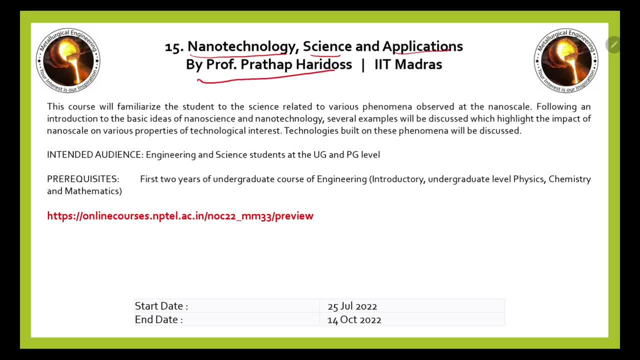 applications. this course is offered by professor pratap haridas from iit madras, so this course will familiarize at the student to the science related to the various phenomena observed at the nanoscale, following an introduction to the basic ideas of nanoscience and nanotechnology. several examples: 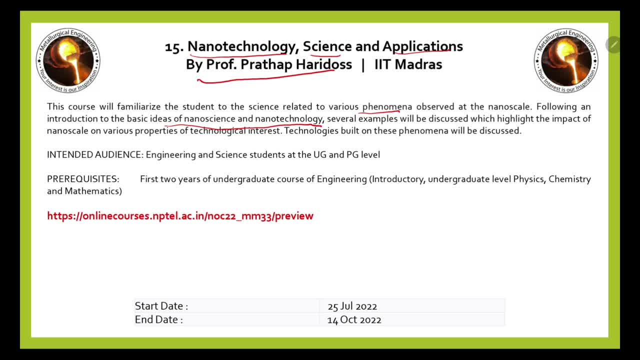 will be discussed, which highlights the impact of nanoscale on various properties of technological interest. so the engineering and science student at the ug and pg level can attend this course and first two years of undergraduate course of engineering, like introductory undergraduate level physics, chemistry and mathematics are the prerequisites of this. 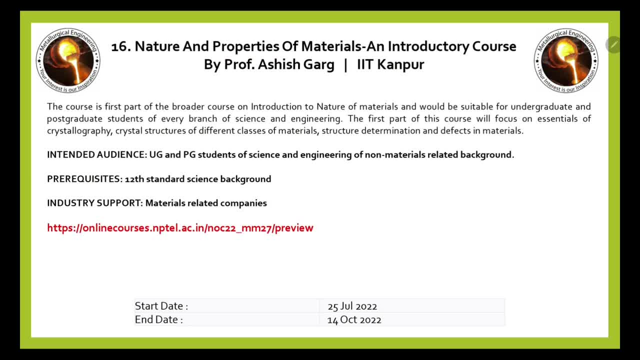 course. next course in this list is nature and property of materials and introductory course that is offered by professor asis garg from iit kanpur. so the course is the first part of the broader course and on introduction to nature of nature of materials and would be suitable. 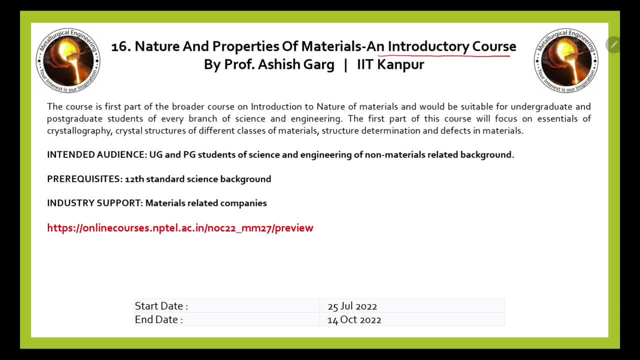 for undergraduate and postgraduate student of every branch of science and engineering. so the first part of this course will focus on essential of crystallography, crystal structure of different classes of material structure, determination and defects in materials. so ug pg students of science and engineering of non-materials related background, if you are from. 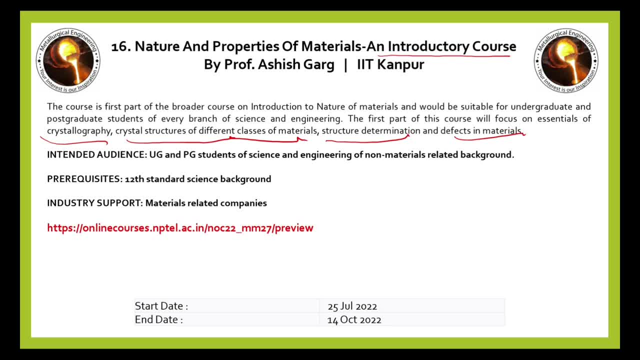 mechanical, electrical, electronics, computer science civil. you are highly recommended to attend this course and know about the nature and property of materials. prerequisites. 12th standard science background is enough to attend this course and materials related companies are also highly recommended to attend this course. course in this list is physics of materials. that is also offered by professor pratav haridars. 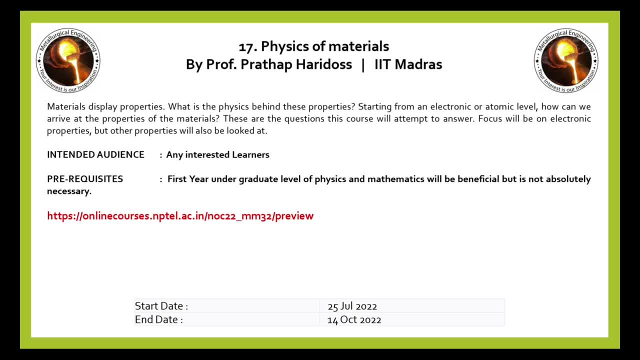 from iit madras. so materials, display property. what is the physics behind these properties, starting from an electronic or atomic level? how can we arrive at the properties of the material? these are the questions this course will attempt to answer. so focus will be on the electronic property, but other property will also be looked at. so any interested? 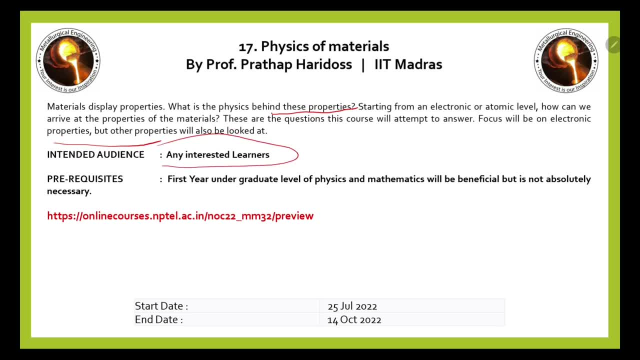 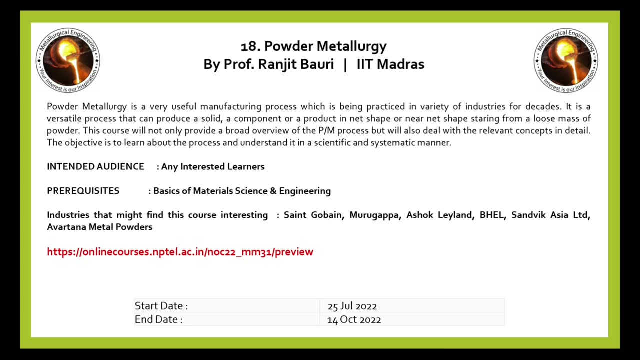 learners can attend this course. so first year undergraduate level of physical and mathematics will be beneficial but is not absolutely necessary. next course in this list is powder metallurgy. this is offered by professor ranjit bauri from iit madras. so powder metallurgy is a very useful manufacturing process which is being practiced in variety of industry for decades. 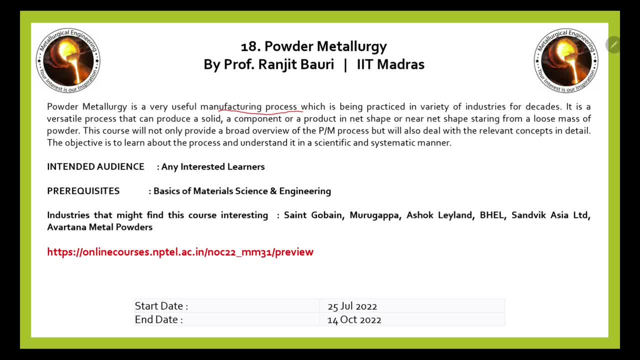 it is a versatile process that can produce a solid, a component or a product in a net shape or near net shape, starting from a loose mass of powder. so this course will not only provide a broad overview of powder metallurgy process, but will also deal with the relevant concepts in 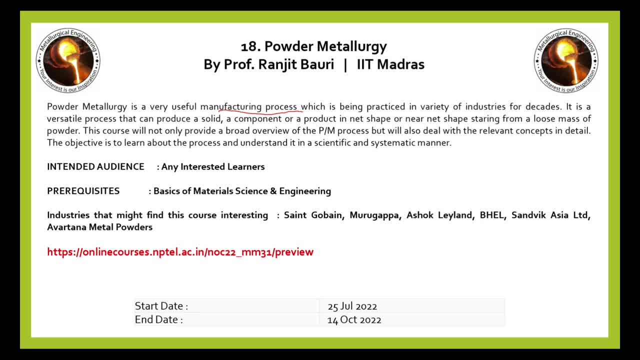 detail. so the objective is to learn about the process and understand it in a scientific and systematic manner, so any interested learner can attend this course. only prerequisites of this course: you have a base. you have knowledge of basic materials science and engineering industry. that might find this course interesting, like saint gobin. 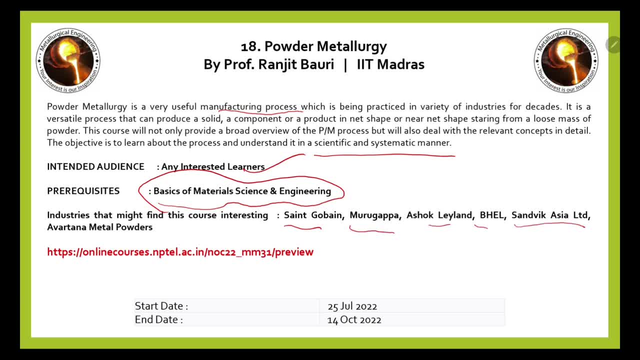 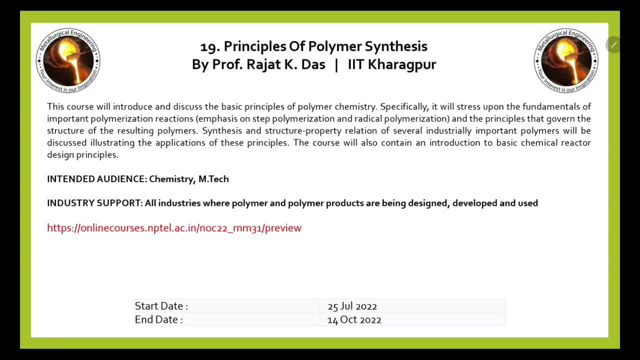 amuruga, asoklil and veil, sandvik asia limited and metal powder. so these are the industry that can highly recommended to attend this particular course. next course in this list is principles of polymer synthesis by professor rajat k das from iit kharagpur. so this course will introduce: 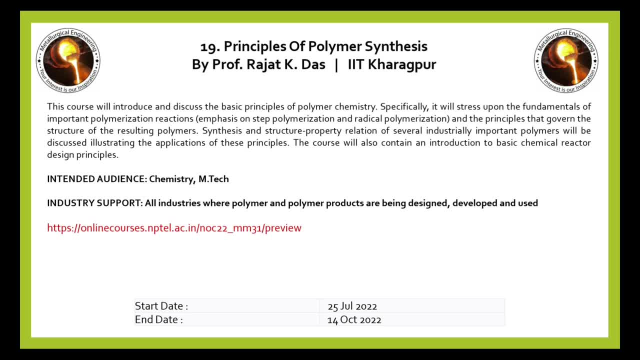 and discuss the basic principle of polymer chemistry. specifically, it will stress upon the fundamentals of important polymerization reactions and the principles that govern the structure of the resulting polymers: synthesis and structure property relation of several industry importance. polymers will be discussed illustrating the application of these principles. so any student which is having 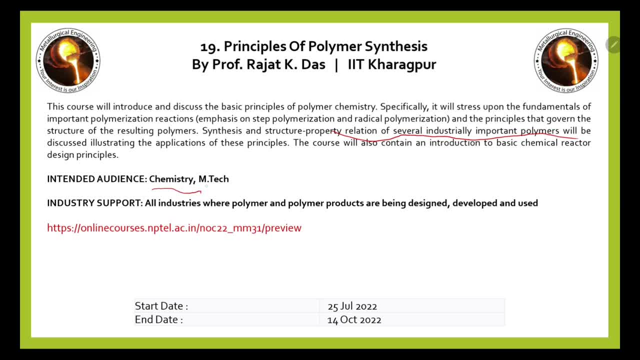 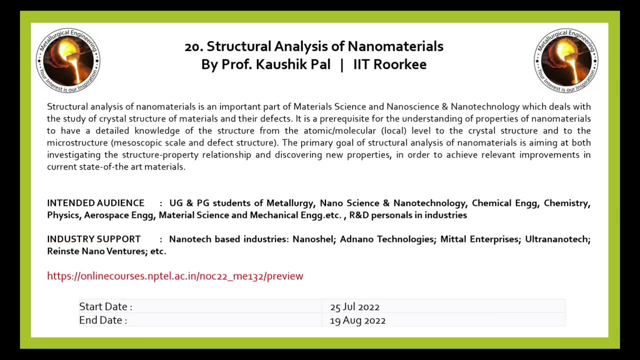 the chemistry background or materials science background, having a mtech degree in materials science, or mtech students in materials science so they can attend this course, and all the industry where polymer and polymer product are being designed, developed and used are also highly recommended to attend this course. so the next course in this list is structural. 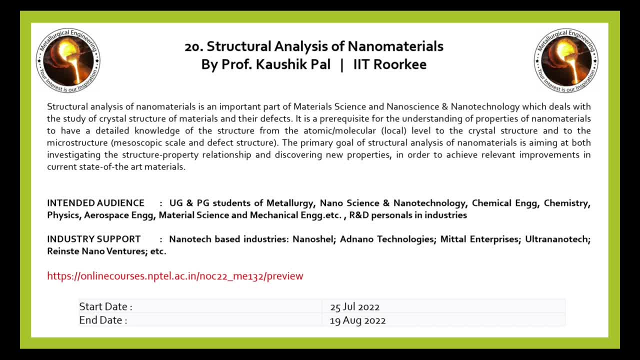 analysis of nanomaterials by professor kaushik paul from iit rudki. so in this course you will try to understand. the structural analysis of nanomaterials is an that and this nanomaterial is an important part of material science and nano of, and nanoscience and nanotechnology, which deals 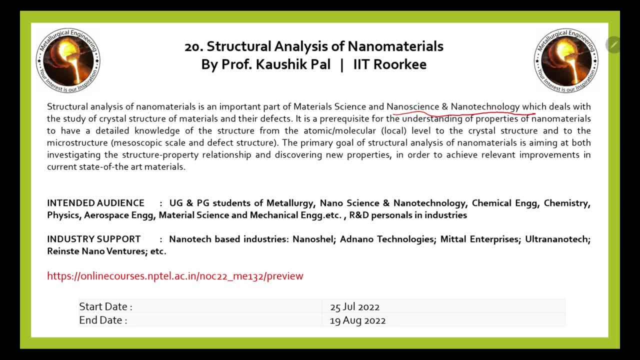 with the study of crystal structure of materials and their defects. so it is a prerequisite for the understanding of properties of nanomaterial to have a detailed knowledge of the structure, from the atomic level to the crystal structure and to the micro structure to this macro level. so the 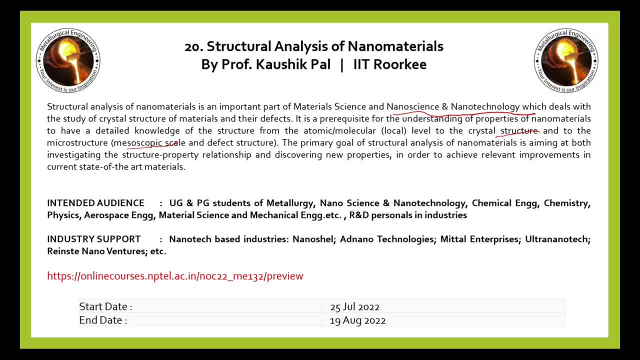 primary goal of structural analysis of nanomaterial is aiming at both investigating the structural property correlation and discovering new properties in order to achieve relevant improvement in current state of the art materials. so the ugpg student of metallurgy, nanoscience and nanotechnology, chemical engineering, chemistry, physics, aerospace engineering, material science and mechanical 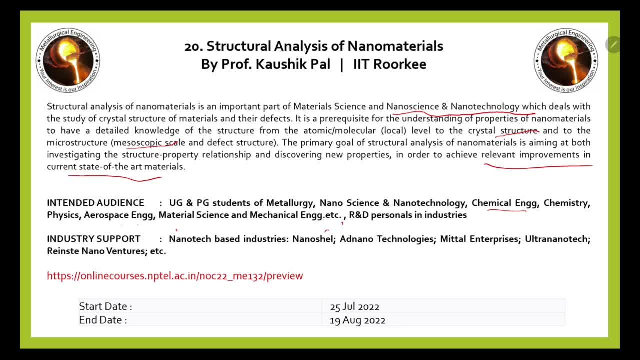 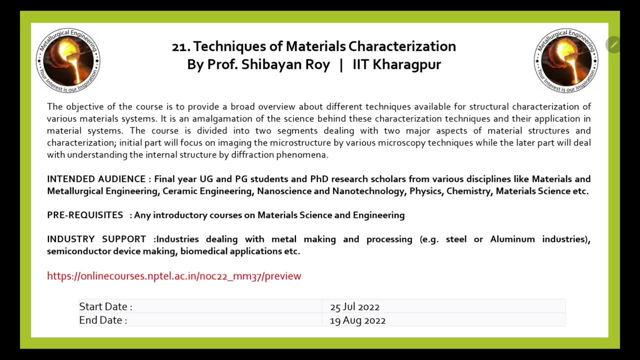 engineering r d personals in the industry- they are also highly recommended to attend this course- and in industry like nanotech based industries, like nano cell, adano technology, metal enterprises, ultra nanotech, mindset, nano venture. so they are highly recommended to attend this course. next course in this list is techniques of materials characterization by professor roy. 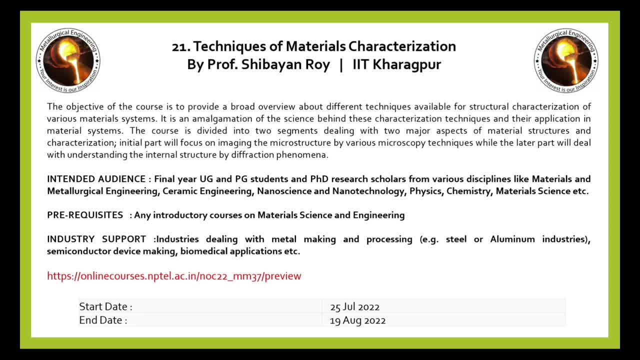 from iit kharagpur. so the objective of the course is to provide a broad overview about the structural characterization of various material systems. it is an amalgamation of the science behind these characterization technique and their application in material systems. the course is divided into two segments dealing with the two major aspects of the material structure and 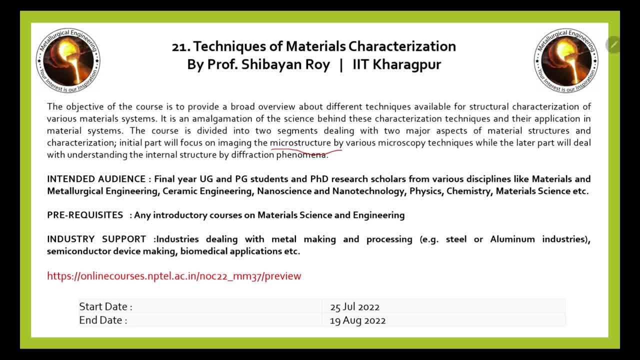 characterization. initial part will focus on imaging the micro structure by various microscopic technique, while the later part will deal with the understanding the internal structure by diffraction phenomena. so in this course you are going to study about optical microscope, sem, dem and also xrd, neutron diffraction. these are the things you are going to study in this course. 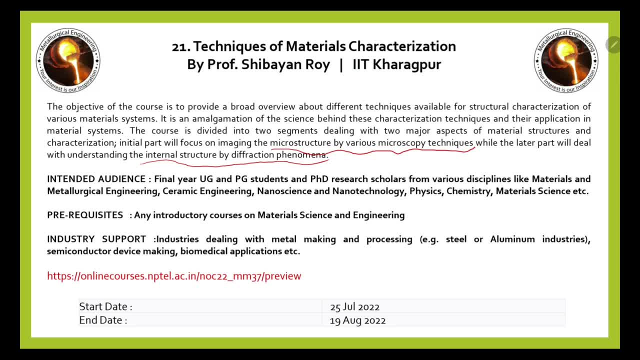 so finally, a ug and pg student and phd research scholar from various disciplines like materials and metallurgical engineering, ceramic engineering, nanoscience and nanotechnology, physics, chemistry, material science are. students are highly recommended to attend this course, and any introductory course on material science engineering is the prerequisites for this. for attending this. 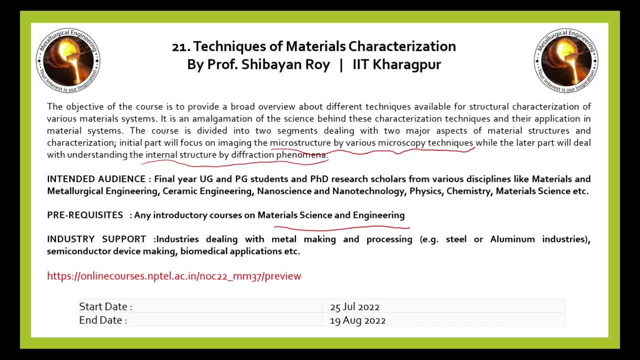 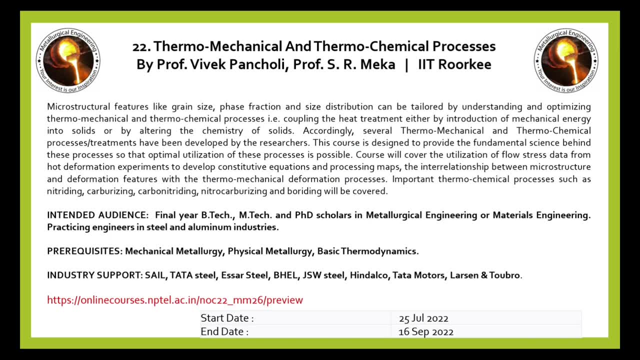 course and industries dealing with metal making and processing, like steel and aluminium industries, semiconductor device making, biomedical application industries, are highly recommended to attend this course. so next course in this list is thermo mechanical and thermochemical processes, offered by professor vivek pancholi and professor sr makeup from iit. so the in this course. so this course is 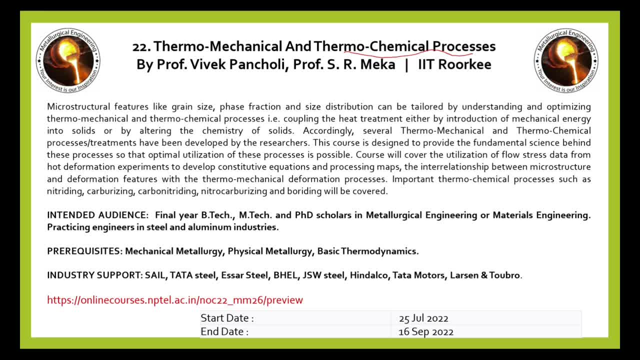 about micro structural features like grain size, phase fraction, size distribution can be tailored by understanding and optimizing thermo mechanical and thermochemical processes. it means coupling the materials of the processes and the chemical properties of the material. so this course is going to be very comprehensive and it is very useful for any kind of chemical engineering. 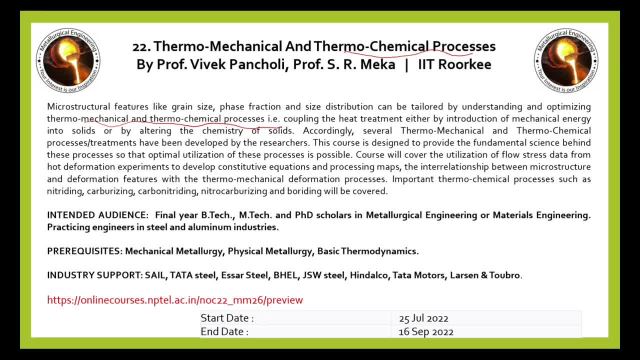 and mechanical processing. so in the next course we are going to talk about the process and how the process is treated, either by introduction of mechanical engineering into solids or by altering the chemistry of solids. so, accordingly, several thermo mechanical and thermochemical process treatments have been developed by the researchers. so this course is designed to provide the 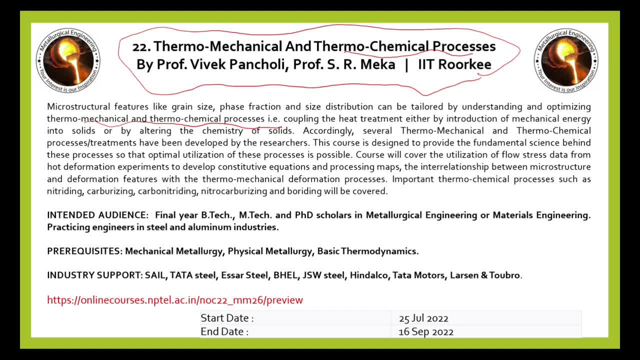 fundamental science behind these processes so that optimal utilization of the process is possible. so this course is highly recommended if you are interested into structure property correlation in this course. So intended audience are final year BTech, MTech and PhD scholars in 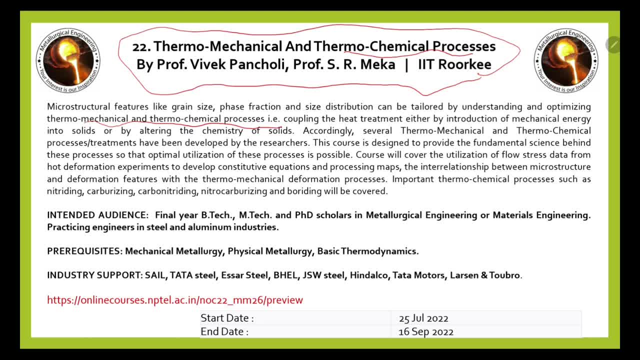 metallurgical engineering or materials engineering, and practicing engineers in steel and aluminium industries are also highly recommended to attend this course. So the prerequisites for this course: you have some knowledge of mechanical metallurgy, physical metallurgy and basic thermodynamics. and the industries like Sail, Tata, SR, Vale, JSW, Hindalco, Tata Motors, Larson and Torbo. 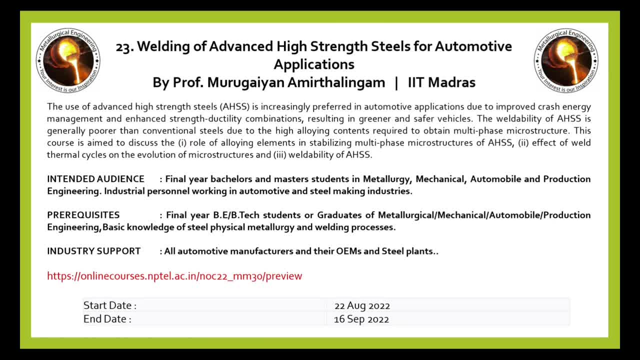 they are also highly recommended to attend this course. Next course in this list is building of advanced high strength steels for automotive applications by Professor Murgan from IIT Madras. So the use of advanced high strength steel, that is also known as AHSS, is 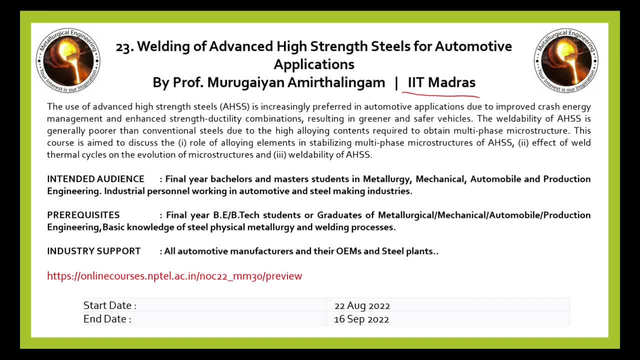 increasingly preferred in automotive application due to improved crash energy management and enhanced strength ductility combination, resulting in greener and safer vehicles. So the buildability of AHSS is generally poorer than conventional steel due to high alloying contents required to obtain multi-phase microstructure. So this course is 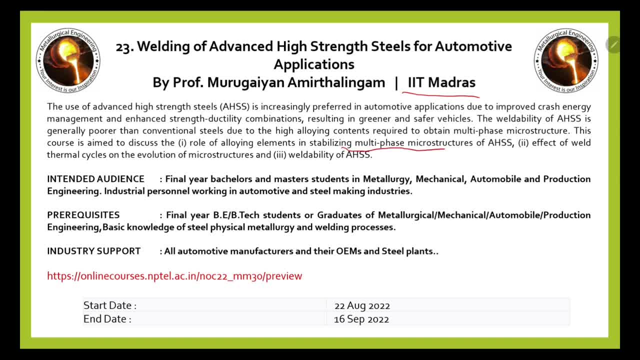 aimed to discuss the role of alloying elements in stabilizing multi-phase microstructure of AHSS. effect of weld thermal cycle on the evolution of microstructure and the buildability of AHSS. So this course is intended audience for final year BTech, MTech and PhD scholars in metallurgy. 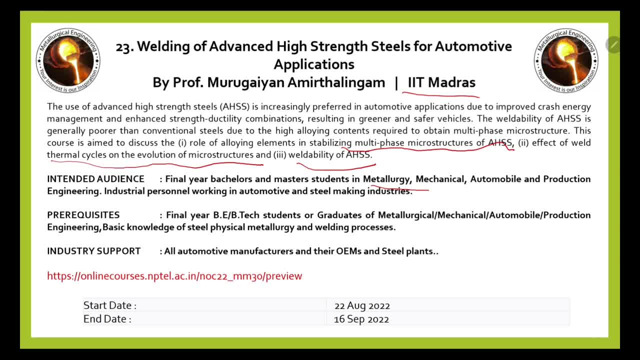 mechanical, automobile production, engineering, industrial personal working in automotive and steel making industries. So the prerequisite for this course is like this. So the prerequisite for this course is like this. So the prerequisite for this course is like this. So the prerequisite for this